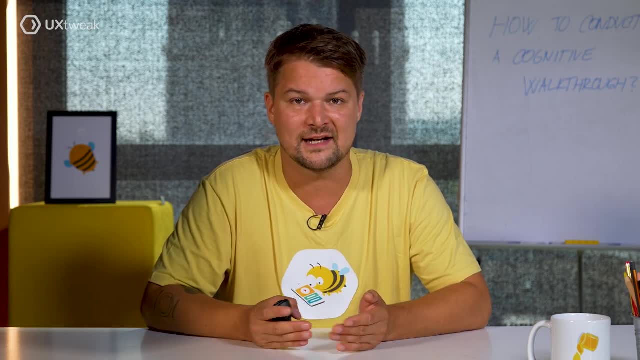 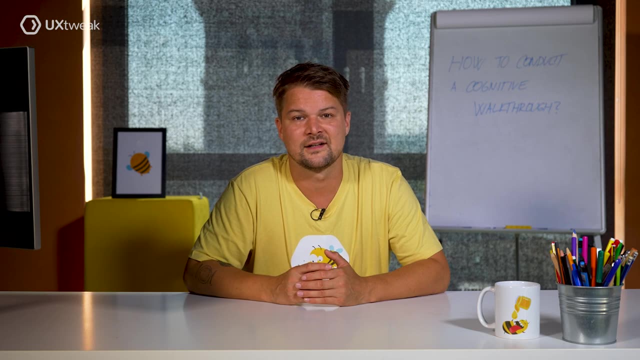 role is the recorder. They record every insight and output of the cognitive walkthrough. The second role is the evaluator. They create a summary after the session is finished. The third role is the evaluator. They are typically the people like UX researchers, UX designers, product managers, engineers and 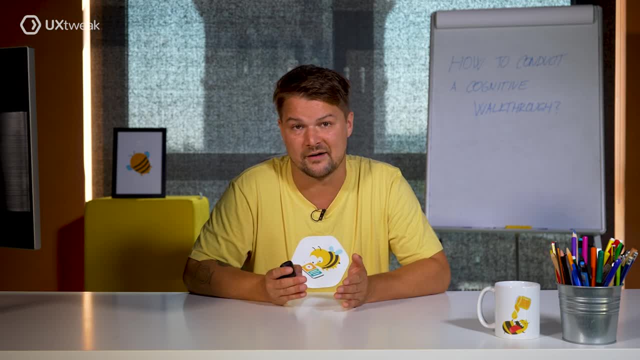 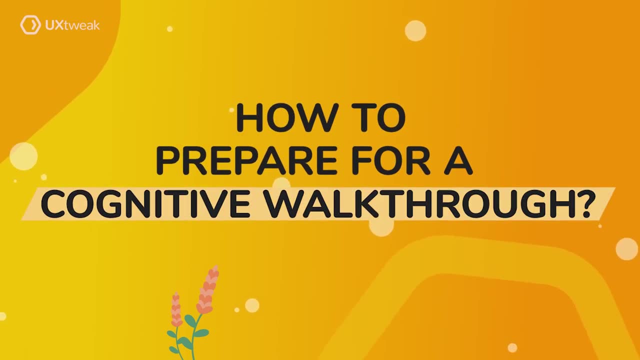 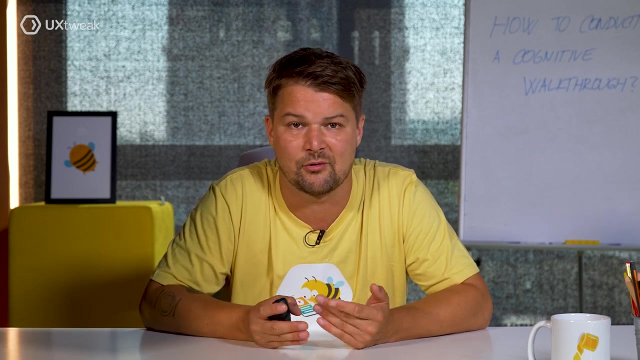 field experts. The more diverse the group, the better, as everyone will have their own unique point of view. The first thing you need to prepare is the prototype. You can create a low fidelity, simple sketch prototype or a high fidelity one in a tool like Figma. 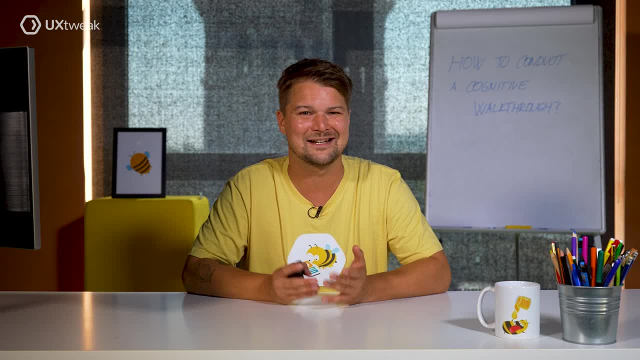 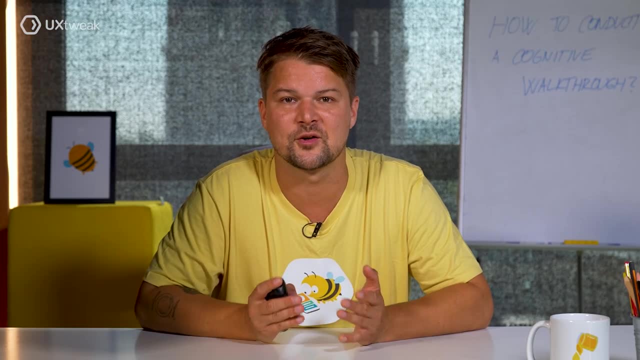 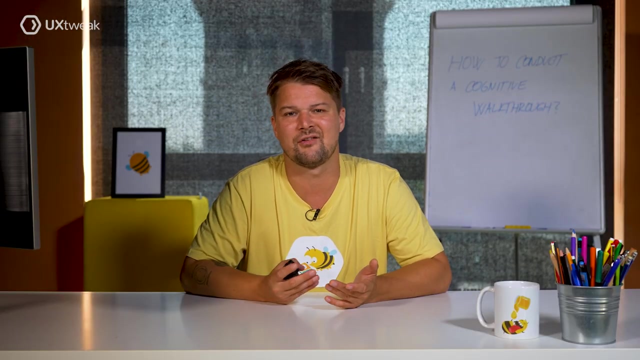 I recommend starting with lower fidelity prototypes to test initial concepts and save the fine-tuned ones for later in the testing process. You should also prepare users' personas you want your evaluators to emulate and the user scenario they should go through. Say you were testing a bike-sharing app prototype. 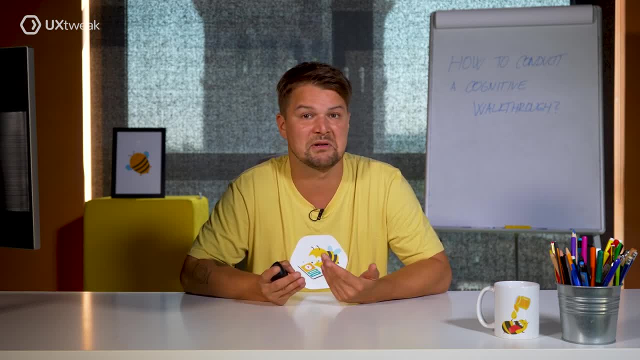 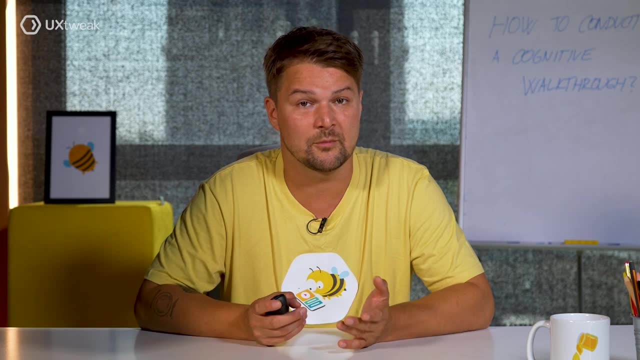 You might define a persona of a middle-aged man- let's name him John- that wants to start riding a bike to work, to get fitter, and is not overly tech-savvy. Your scenario could be this: John registered and wants to borrow a bike. 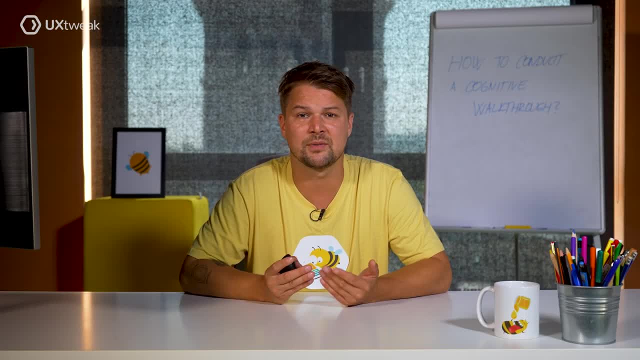 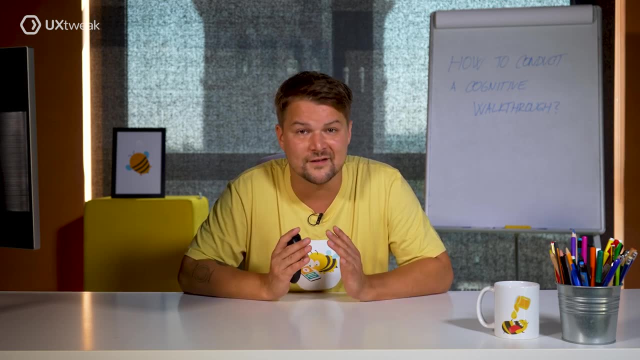 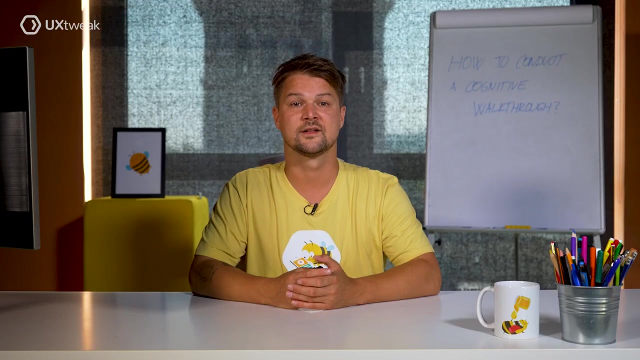 for the first time. How is the process for him? Another scenario could be completing the registration of process itself. You can conduct multiple cognitive walkthroughs for different personas and scenarios. So you have the prototype prepared and have gathered your group. Now what? 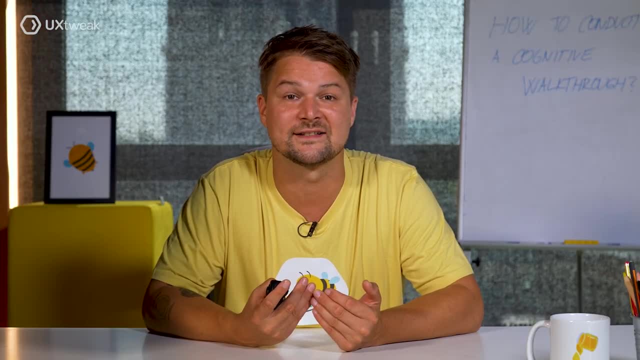 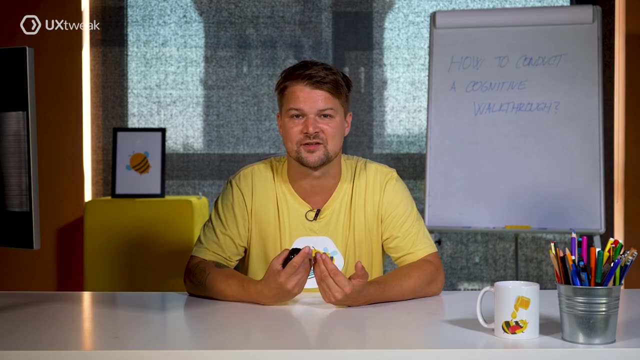 The first step is for the presenter to describe the chosen user persona and scenario to the evaluators in as much detail as possible. They have to adopt the mindset and situation of this persona, so make sure not to overlook this step. Once the persona and scenario are clear, 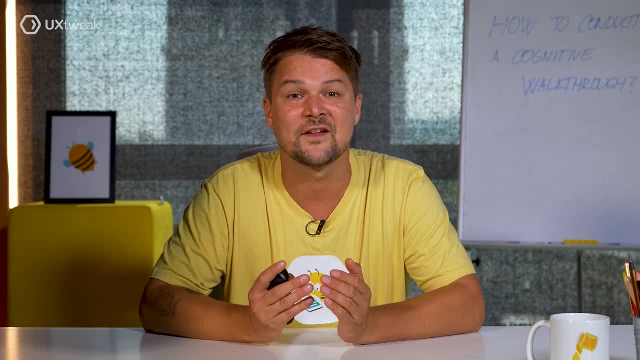 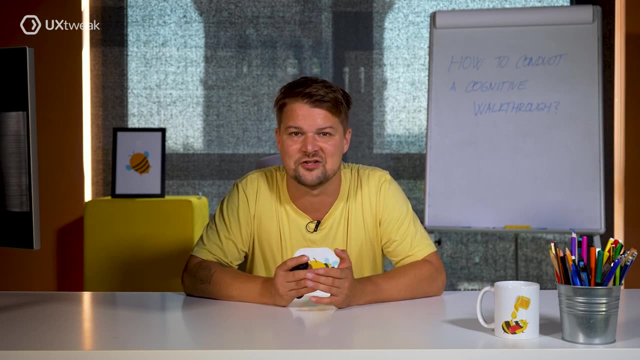 bring forth the prototype and the group can start discussing the first action the user would take to accomplish their goal. There are four defined questions to help assess every action during the cognitive walkthrough. These are: will the user try to achieve the right result? Will the user notice that the correct action is available?